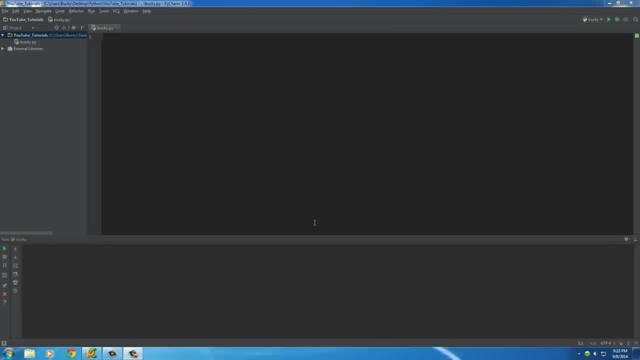 Alright, guys, welcome back to another tutorial, and in this video I'm finally going to start talking to you about classes and objects and some cool things that you can do with them. So first of all, what the heck is a class? Well, the most simple definition is basically: a class is an easy way where you can group similar variables and functions together. So say you're making a computer game, Usually all of the functions dealing with enemies and all the variables to utilize. 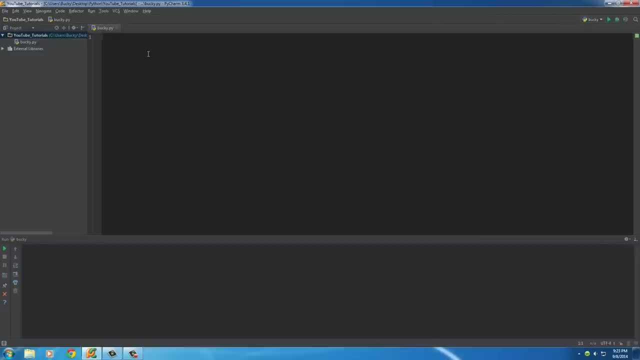 You want in an enemy class. Maybe you have a different one for moving your character around. Well, all of those functions for moving your main character would be in a character class, So on and so forth. So again, the most simple definition is: it's a really cool way where you can group similar variables and functions together. Might have been recording. Okay, just checking. So, with that being said, let's go ahead and look at an example right now. So, in order to make a class type, the keyword. 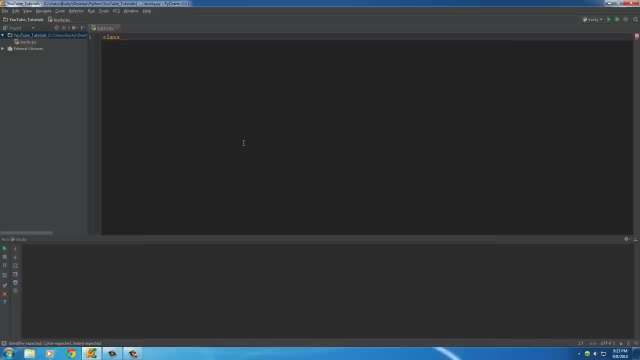 class and then add a space. Now class pretty much says: hey, Python, I'm about to make a class. Now, after this, what you want to do is you want to name your class something, and it's common practice to name it with a capital letter, And this is just so programmers can differentiate between a class and like a normal variable or a function or anything like that. So this is how we make a class called enemy. Now add a colon, Now whatever is indented. 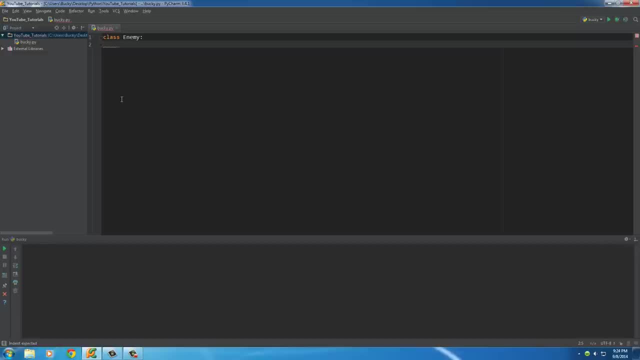 after. this is going to be part of your enemy class. So every variable inside here and every function is going to belong to this enemy class. So let's go ahead and make a simple variable first. So we'll say that each enemy has a life of three. So now this life variable is actually part of this enemy class. Just remember that. So now what we can do is we can make a couple functions for this class. So what's one of the 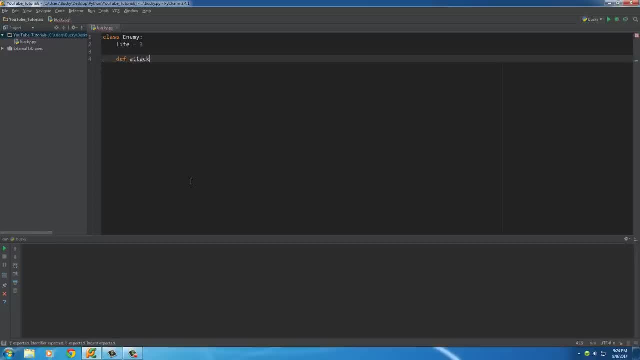 things that we can do. We'll say we'll make a function called attack, and this is just what happens whenever we attack an enemy. Now, check this out Whenever I'm just writing these parentheses right here: what PyCharm did, is it automatically filled in this keyword of self? Now, this is going to be a little confusing until I finish this program and explain what objects are, But pretty much, think of, whenever you see self, it means 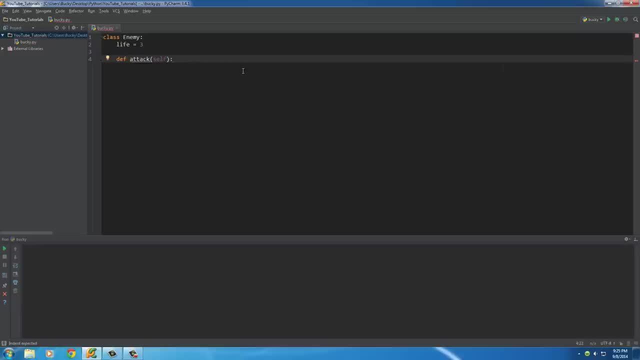 use something from this own class. So if you say you're going to see later like self attack, it means use the attack function in this class. Self life means use the life variable in this class. Again, kind of confusing at first, but you guys are going to see later on what it does. Alright, so let's make this function actually do something. Whenever we attack the enemy, we'll just do something like print attack or actually let's print ouch. We'll say that the enemy says ouch And then we'll say 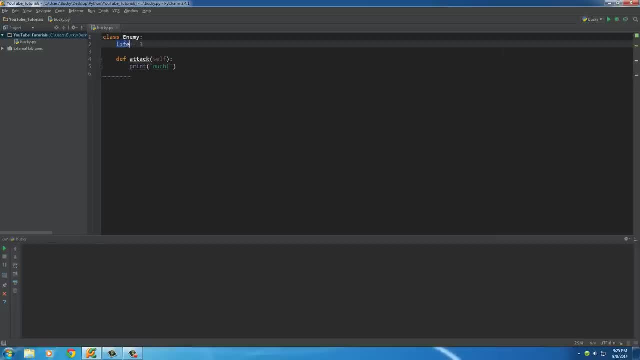 and also what we want to do is we want to subtract one from the enemy's life. Now, we can't just do this, Check it out. If we just try to subtract one from life, we get a little error. What we actually need to do is what I was talking about: put self life So that's how you access the variables inside your class. So pretty much self is saying: okay, inside this class, take away one from the life variable. 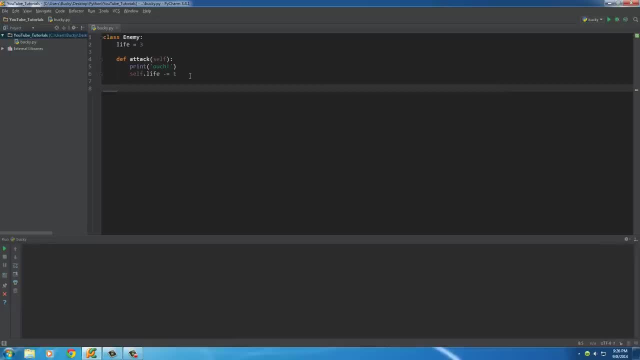 Simple enough. Maybe it was easy. I don't understand Who knew. Alright, so let's make one more function. so this class isn't that boring. We'll make another function to check the enemy's life, And of course it automatically fills in that self variable And we'll say, I don't know, maybe a little if statement, So if self not slough, So if self life is less than or equal to zero. And this is actually another. 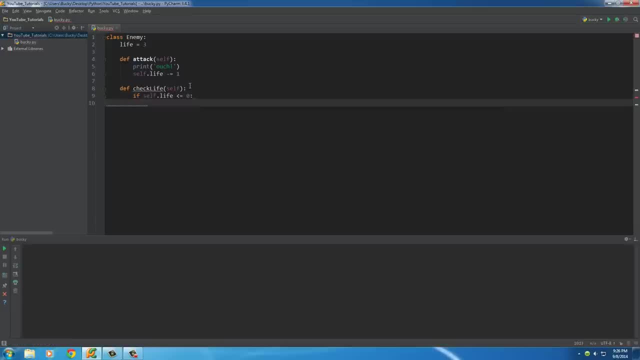 thing I want to point out: Whenever you're making computer games, don't just check if the enemy's life is equal to zero to see if they're dead. Because like, if they had three life and you had, like a super powerful weapon to like slash them and it took away five life, Well then their life would be negative too. So always make sure to check if it's less than or equal to zero. Just a little, I don't know tip for game development. So if they're less than or equal to zero, we'll just print something, like I am. 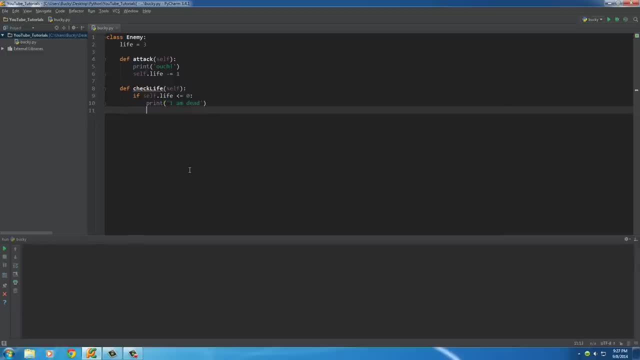 dead. The enemy obviously couldn't say anything if it was dead. But this is our game. We can do what we want. Alright, so if they're dead, they're dead. Else we'll just print out like how much life they have left. So print something like: of course we need to convert to a string. So print out the amount of life that they have left And we'll just do something like: this Life left. 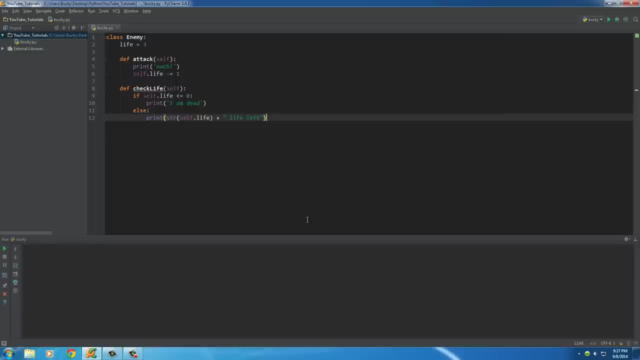 Like two life left, One life left, Tomato, Tomato. Alright, so right now we have a very simple class of enemy. So the enemy has three life and we can attack him. Whenever we call this function, it takes one life away. And also, anytime we can have it, check to see how much life the enemy has. If it's dead, it prints out I'm dead, Or if it's not dead, it tells you how much life he has left. Simple and easy. 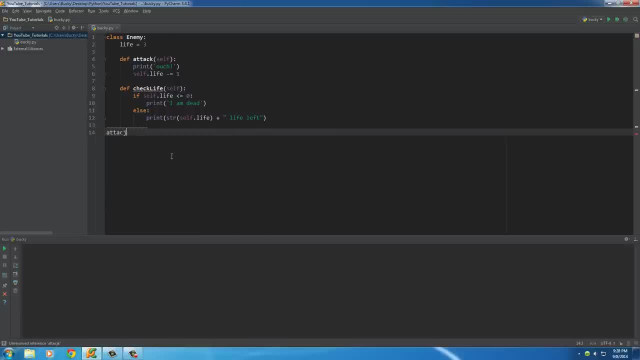 Now, if we just try to do something like this, Attack, Okay, well, that's not working. Now, the reason that this doesn't work is because, in order to use anything inside your class, you need to access it a special way, And that is by creating something called an object, Now, an object. just think of it like this. It's pretty much a way that you can access the stuff inside your class. 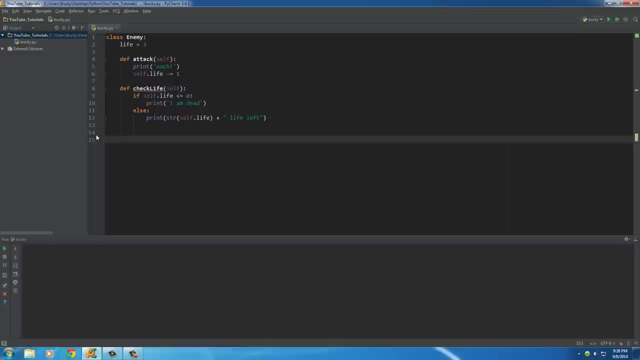 And I know I just said that twice, but it's actually really important to understand And they're really easy to make as well. So the first thing you do is you pretty much act like you're making a normal variable. So I'm going to make an object called enemy one. So what you set it equal to is the class that you want to use stuff from. So I want to use the stuff inside the enemy class. So anytime I want to use that, I need this object. 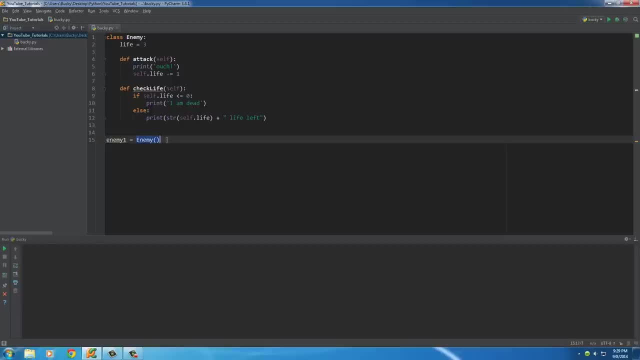 Called enemy one And it's object from this class right here. So now we can just do something called enemy one Attack. And what this pretty much means is this: It says, okay, enemy one is an object from what class? Well, enemy. So go to the class enemy And once you're in there, use attack. So now, if we just 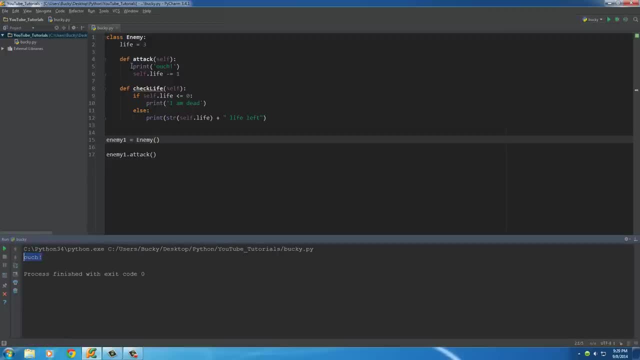 try to run this, It would say ouch, because it just took one away from the enemy. And actually, if we check life to make sure that worked, Whenever we run this, It said: okay, it starts with three of course. So we're going to attack this enemy once. Say ouch, Then it says two life left. Now I want to show you guys one other really cool thing, And this is probably. 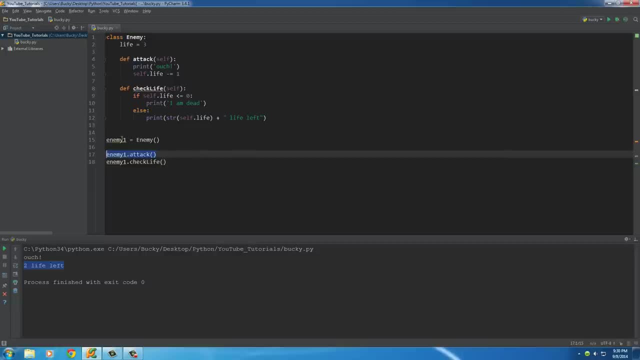 the main reason that people use classes all the time. See, each object is actually a copy of its class, So each object is actually independent of one another. So check this out. Don't understand what I mean. You will, in just a second, Say that we have enemy one And say we have another enemy called enemy two. Actually, let me code this entire thing and then I'll talk you guys through it. 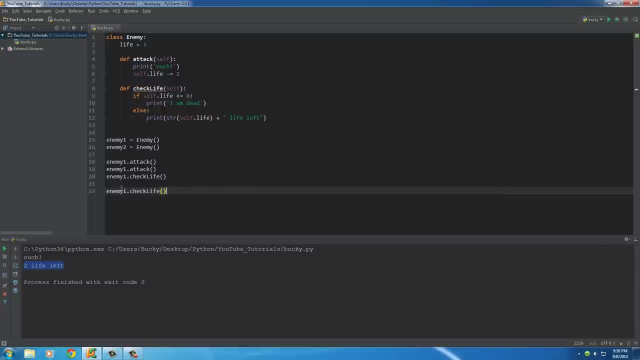 And let me do this Alright. So what's going to happen is we're going to make two objects or two copies from this class. One of them is going to be stored in the object enemy one And another one is going to be stored in the object enemy two. Now, each of these are pretty much think of them like their own enemies, So each of those has three life each. So whenever you